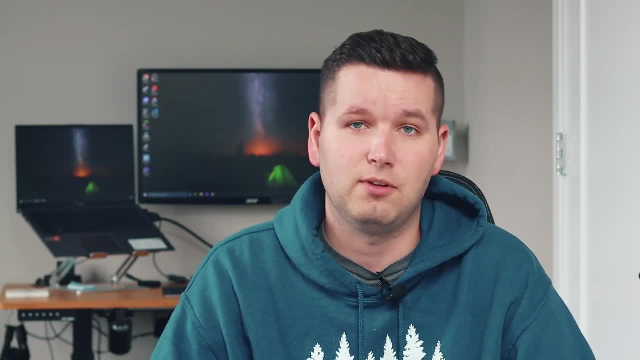 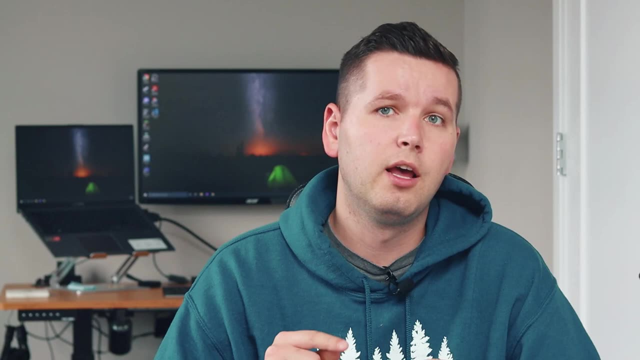 programming and hence why I'm recommending C is the first language to learn. you want to master it, not just like, hey, I did hello, world program, I'm good to go now. you want to really understand. how do the pointers and addresses work? how does my program work and how does my software program work? 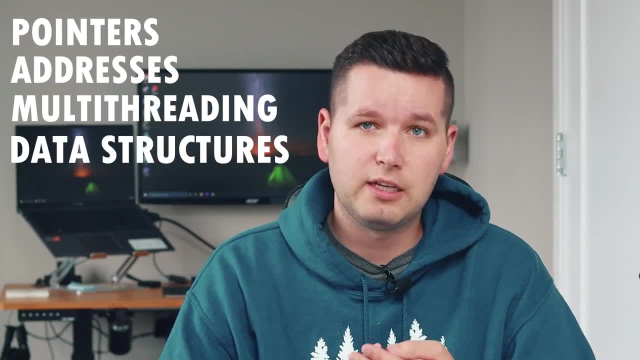 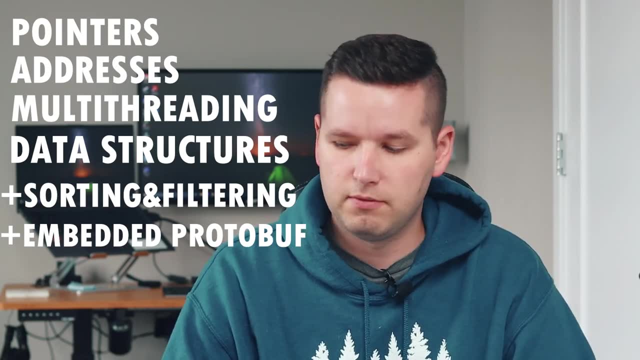 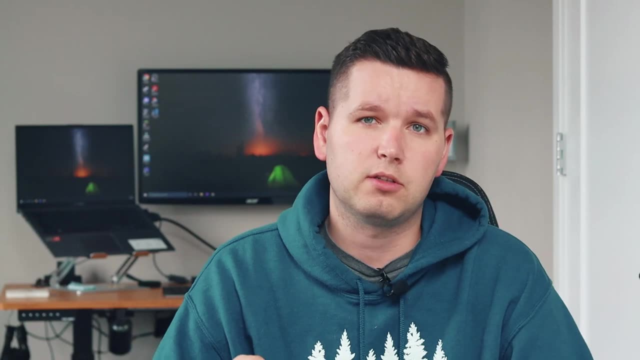 multi-threading work in C programming and you want to learn about data structures as well. so those would be the general topics you would want to understand, at least by minimum, be very proficient with them, understand how to do work, which methods are faster, what is slower. those are really important parts. 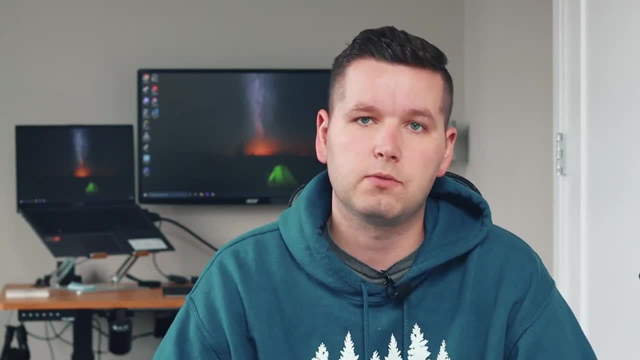 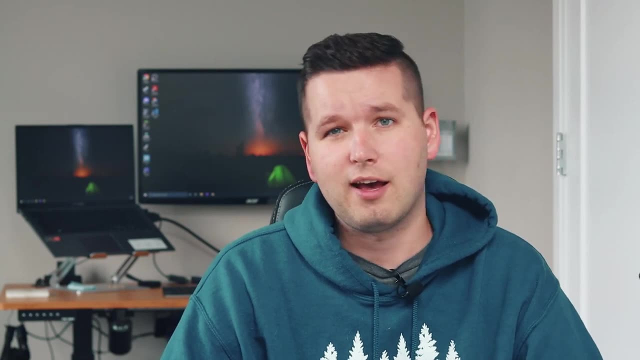 in in any programming language. you you want to optimize your software for the best performance or best power efficiency, so you would, you would want to keep all these things in mind. later on, you can add on to languages like C plus and Python for later on, but honestly, focus on C first. that that would be my 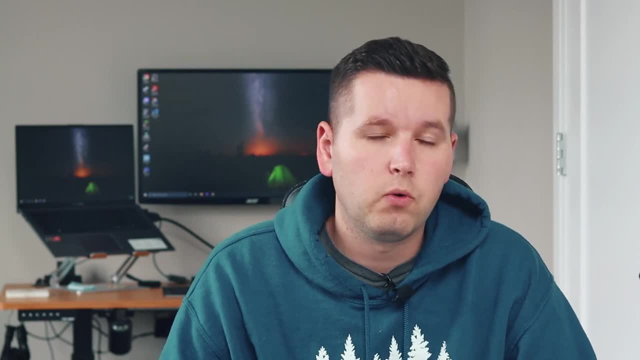 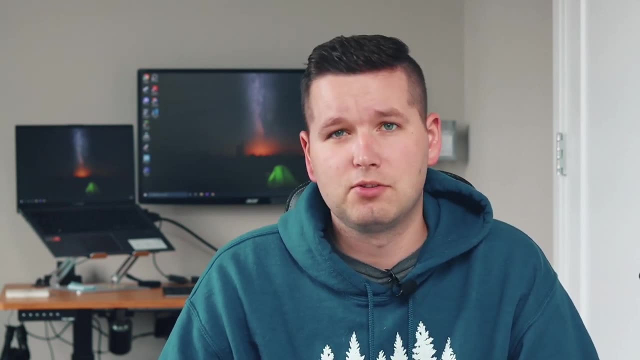 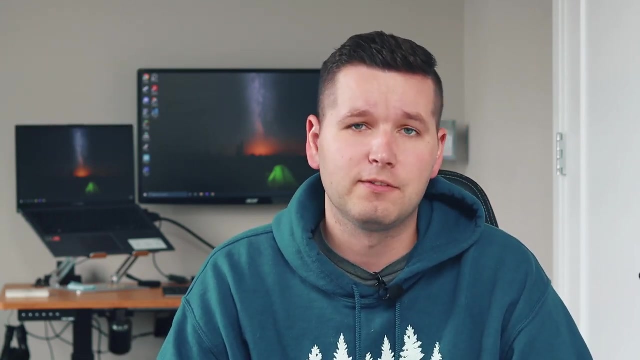 go-to. there's plenty of C programming tutorials on YouTube, so go ahead and search around, look for good reviews and so on, for things that would get you going. essentially, initially, just follow the tutorials and then move on to a project mindset. you don't want to just blindly follow tutorials all your life. 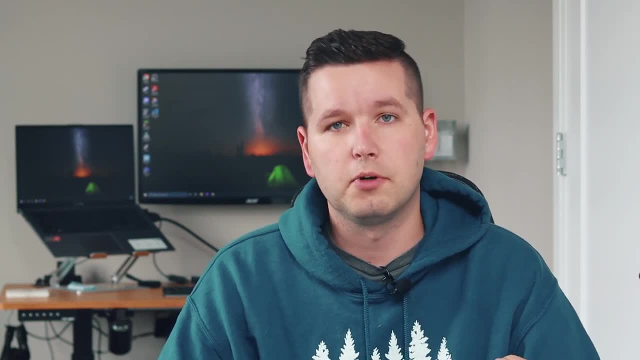 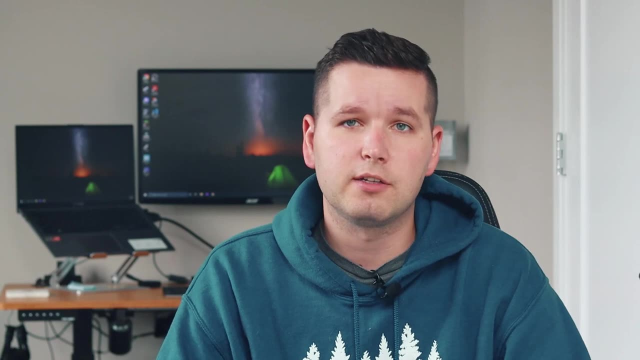 you want to develop this concept that, yes, you were able to go through the tutorials, learn things, but now you can apply the in real life by yourself. so come up with projects that you think you would enjoy and make sure you can actually execute them and go, go ahead and challenge. 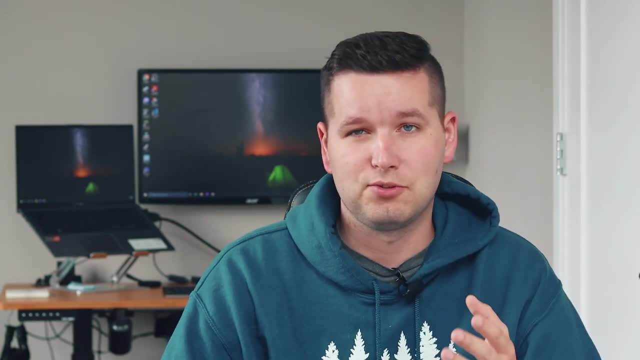 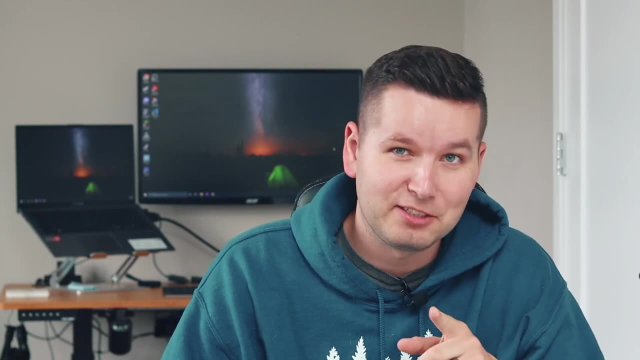 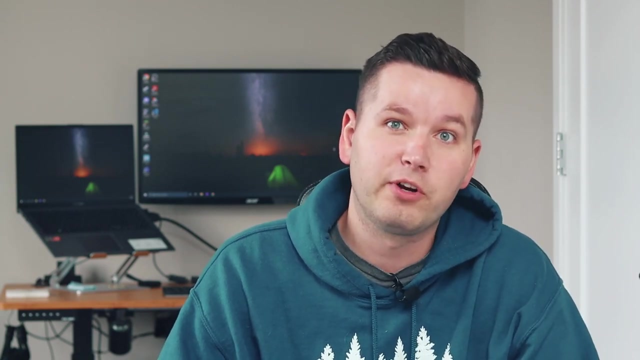 yourself to do those projects so you can learn and practice your C programming skills. well, now that you have mastered C programming- which I know you slackers did not do that, so you guys just jumped into the second point- we're like: okay, yeah, I know I, I saw a tutorial five years ago about C programming, so I'm 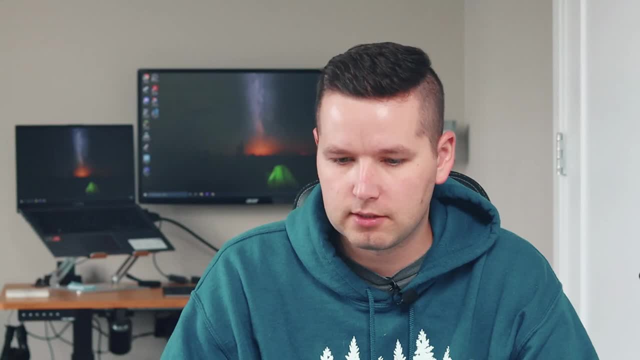 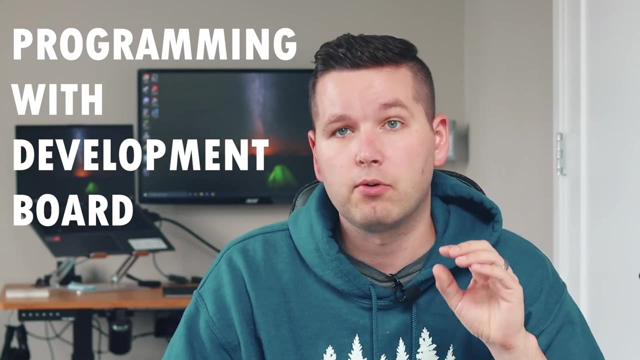 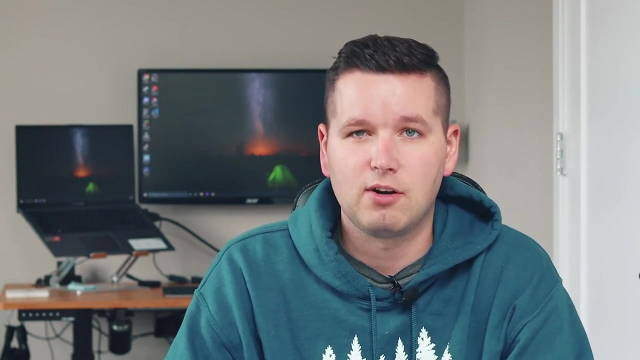 good to go now, but anyways, you you need to move on and start start doing things on a development board. so that's where actually the embedded software program comes in, where you start program the microcontroller and you will make it do things that you want it to do. I think the best place to start would be like: 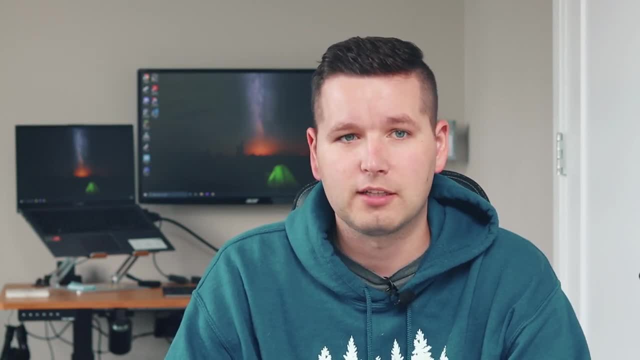 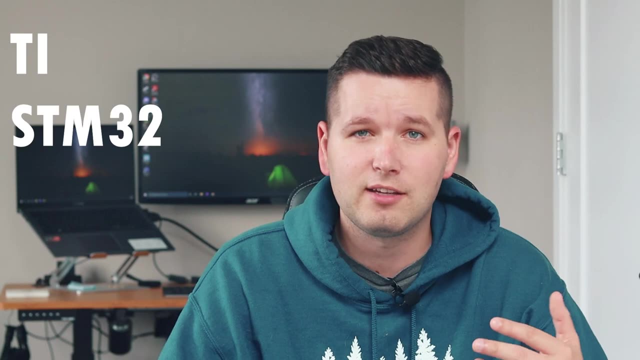 Arduino or Raspberry Pi if you really want to learn that like about like the basic stuff. but if you're not already familiar with those things, if you're already familiar, I would recommend looking into, like TI and STM32 or something that, to get those development boards. and I'll list some development. 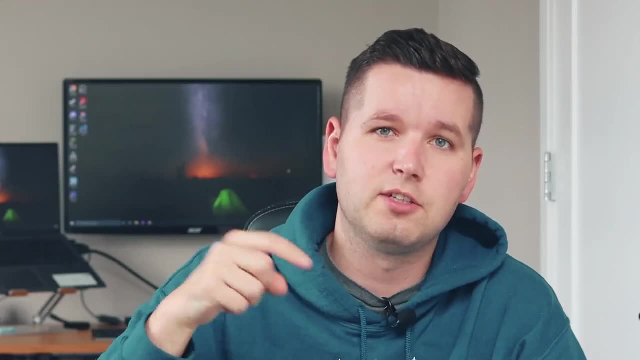 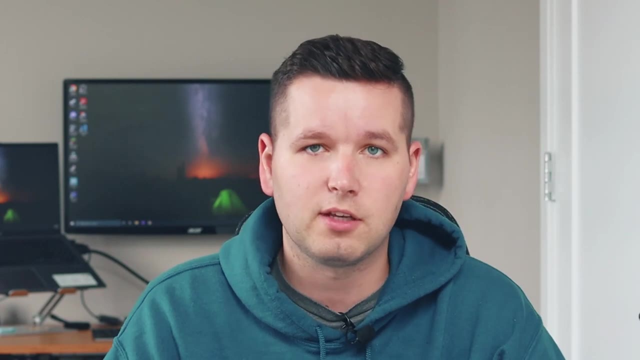 boards in the comment section below, so go check them out. they're just links to Amazon and you can purchase them. and if they're their affiliate links, so if you use them and you buy something on Amazon from that, that's the way you can support this YouTube channel as well, the reason why I really recommend that Raspberry. 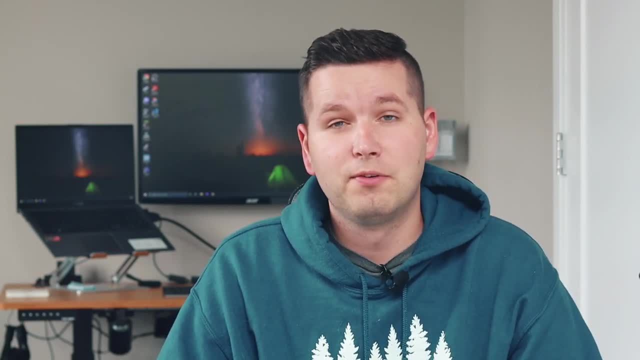 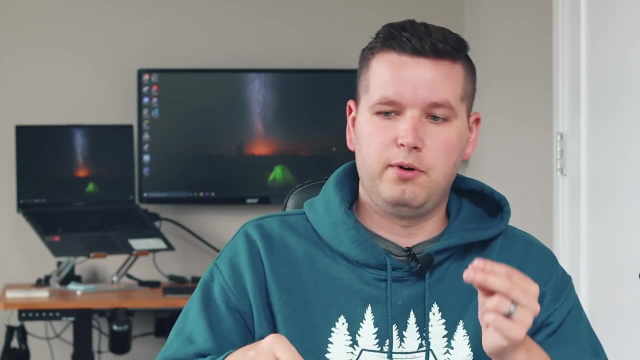 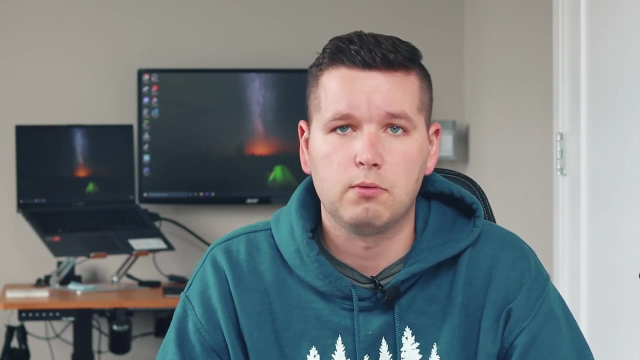 Pi and Arduino is because they have so many projects available for free for and like. they're great tutorials. they literally will show you like how to connect things on a breadboard and like make these connections and how to connect these sensors, and they give you an example code and you can do your own stuff with. 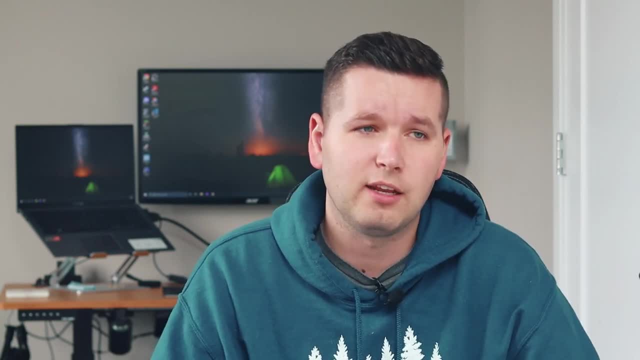 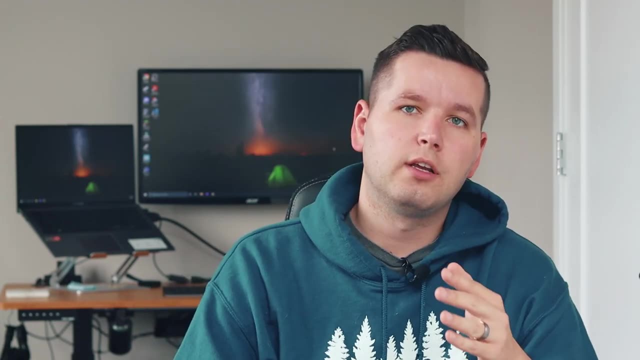 it. I think that's really helpful and beneficial, especially in the beginning, for you to develop understanding how things work and how these sensors interact with a development board as you're starting off to do your projects on the development board. during that process, you want to learn about things. 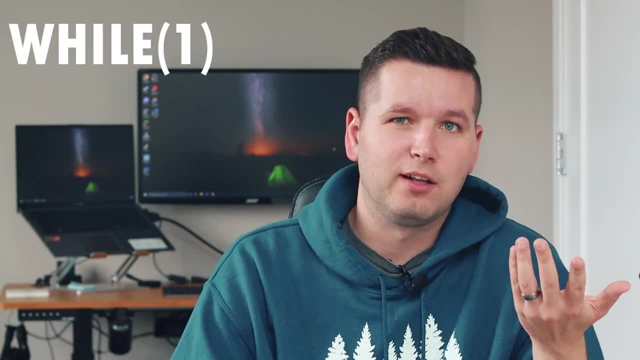 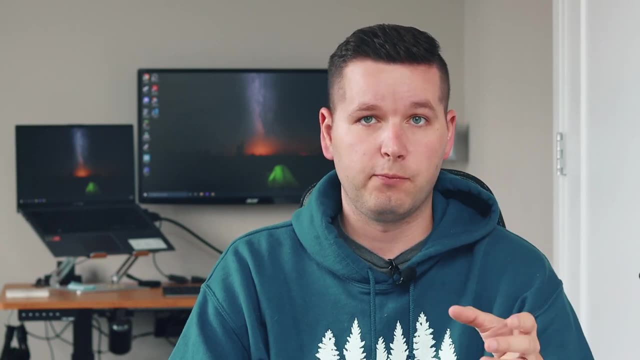 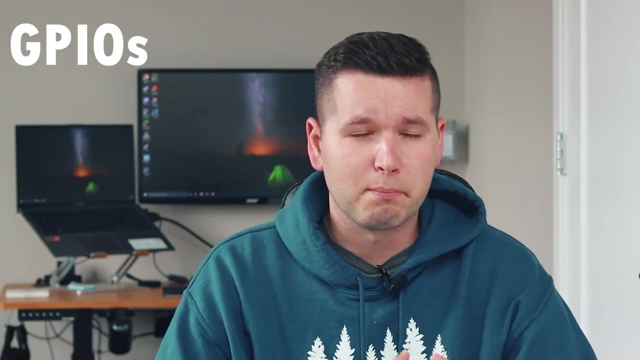 like super loop or a while of, really a while of that's. that's really like the easiest way you can do embedded software programming. you will have this loop that will stay in it forever and it will execute things that you would tell it to execute. next is like you want. you want to learn about GPIOs, like how the 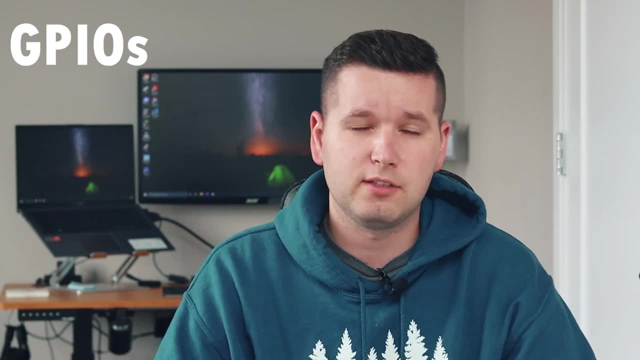 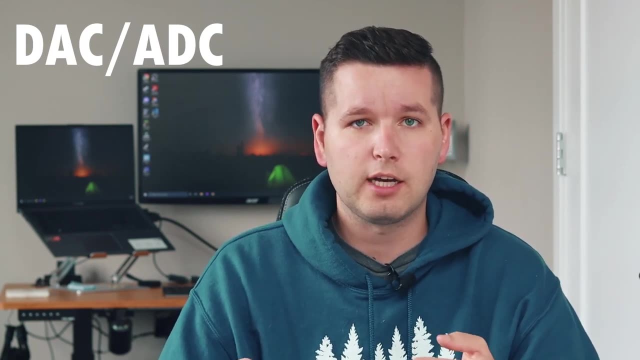 buttons, switches and LEDs work, so those are probably like one of the first things you will learn. next one is like digital to analog conversion and analog to digital conversion, and again, those are one of the main topics that you will need in order to use sensors or use analog sensors or send out a 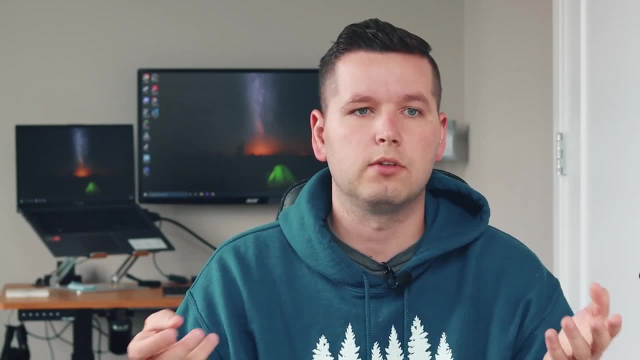 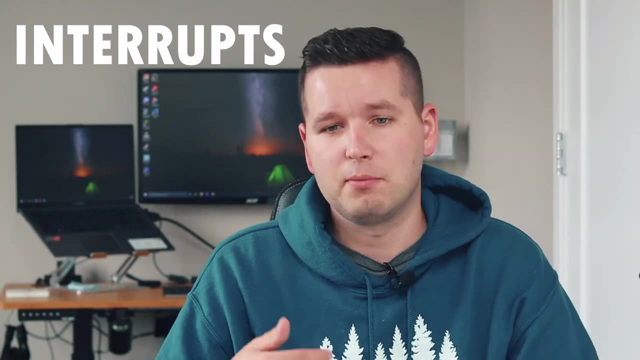 digital signal that you need to convert to an analog signal in order to make something happen. the next concept you want to learn about is interrupts. it's highly important, so, and it's very commonly used. you want to make sure you understand how it works on the development boards. honestly, if you 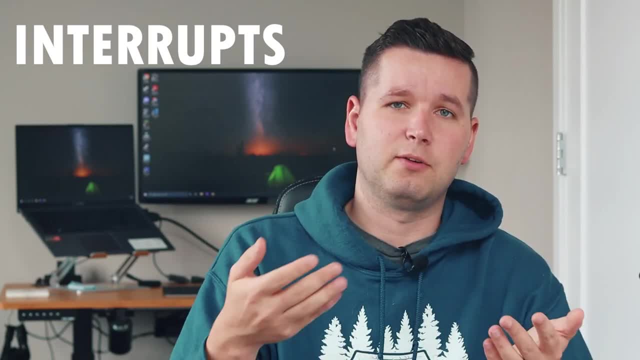 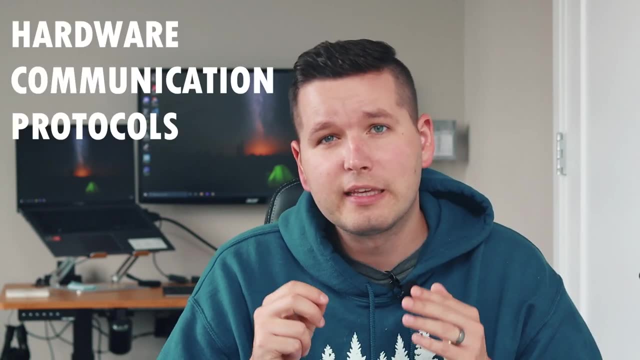 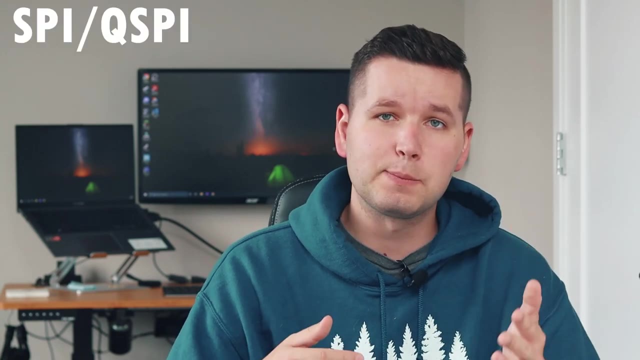 learn in one development board. kind of the concept is to save on other ones. so just just having a general grasp of how things work on that would be very important. next up is communication protocols, and this is this is a big one. this is highly commonly used, but the main ones are like SPI, QSPI, SPI as serial peripheral. 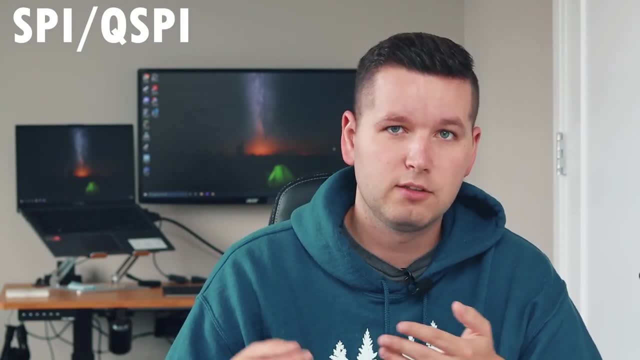 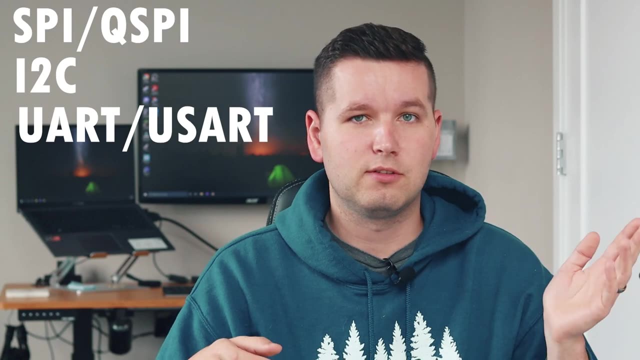 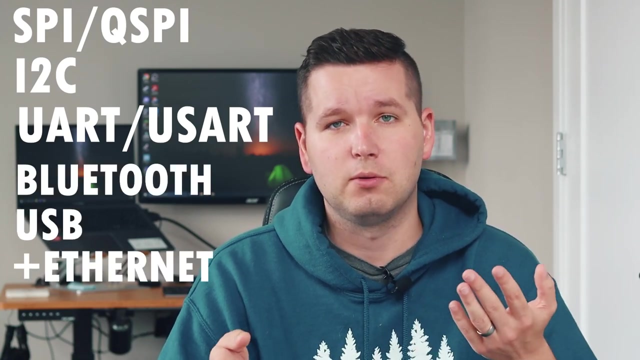 interface, or QSPI, which is quad serial peripheral interface, and then you also have I2C, then you have UART. you also have USART, which is the synchronous or asynchronous version of UART. so there are more advanced concept like Bluetooth and USB that you would also want to learn later on. next up is DMAs, which 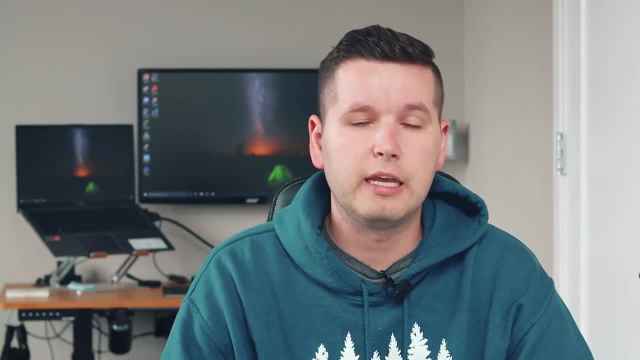 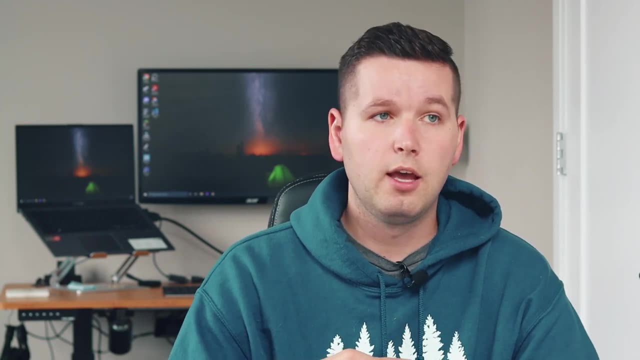 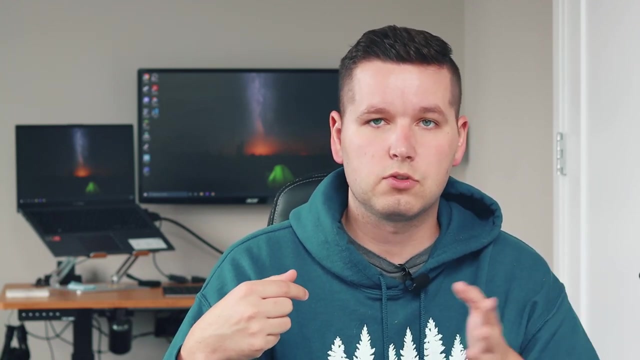 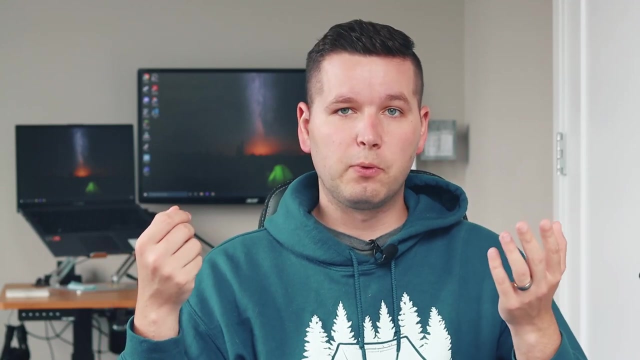 really is huge, huge for for any data processing. it allows you to have a single core system and you can say to the CPU that hey, set up a DMA to using an SPI to collect- they constantly collect- data from this external sensor. while that DMA is collecting that data into this specific memory location, the CPU is free to do. 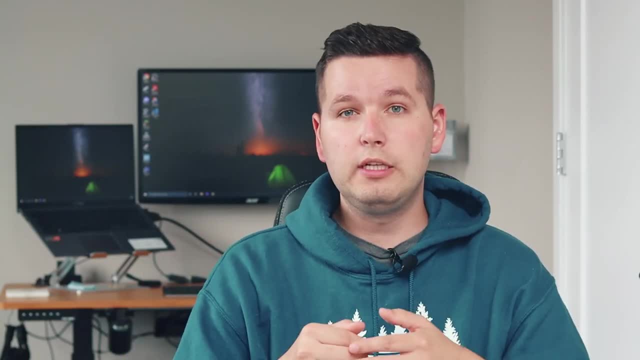 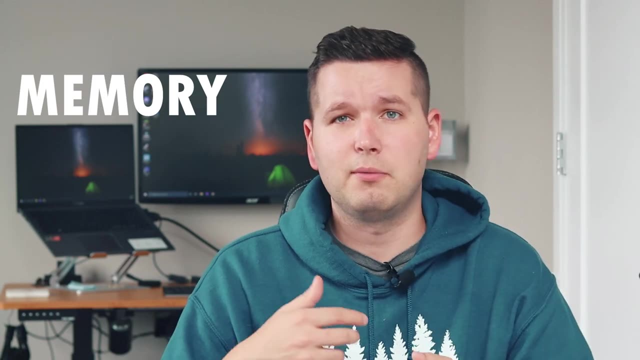 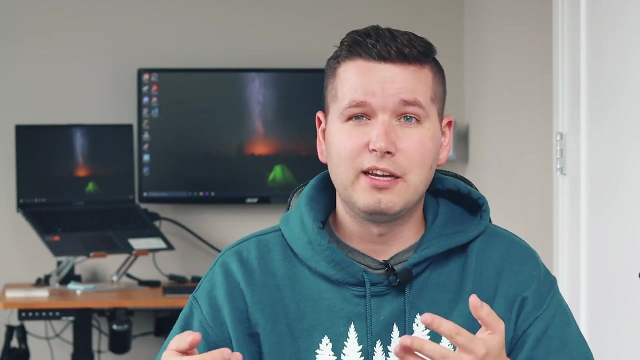 whatever it wants, so it's not held up by anything else, so it really drastically can reduce CPU overhead. well, next up would be memory management. so you want to learn about how a simple flash memory reads and writes work, so, and later on you can move on to DDR memory. next up is RTOS. 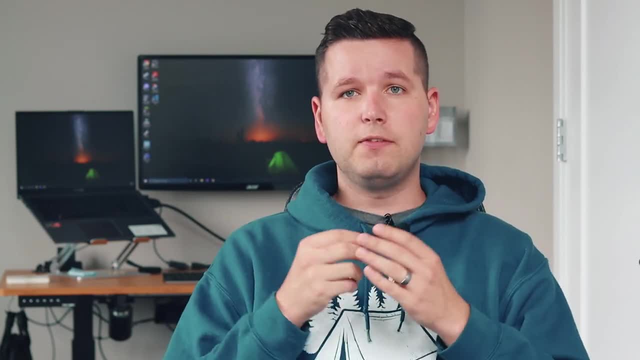 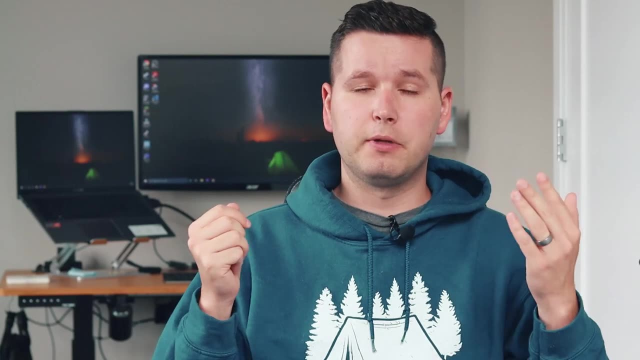 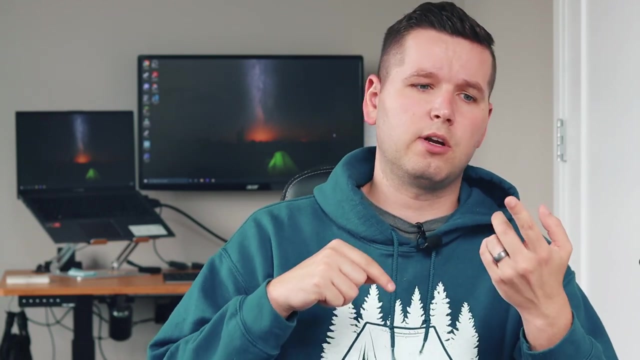 system, which is real-time operating system. so you definitely want to learn about this and how it works. you don't have to go into these crazy concepts. but again, this is why I was telling about: you want to learn about how multi-threading works, how does semaphores work? how does 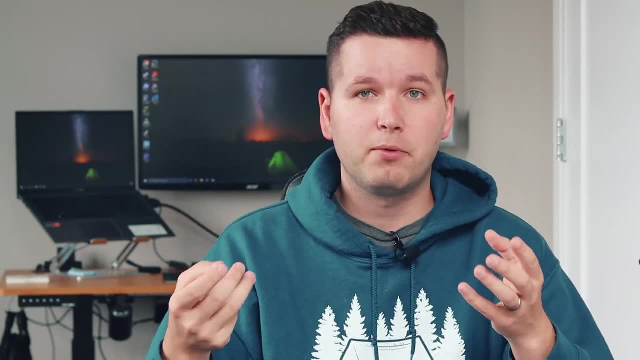 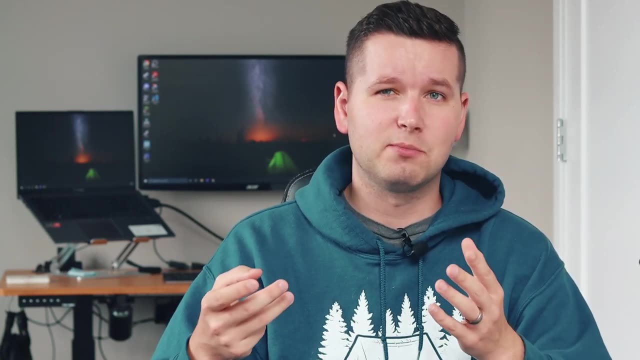 threads work. so you, you want to have that understanding of operating systems. so if you're in a university or you're you're taking an online course or something like that, an operating systems course would be a good recommendation from me. honestly, you would probably for embedded systems, you would want to focus. 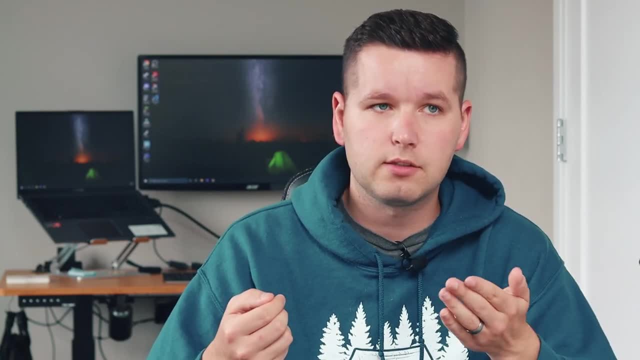 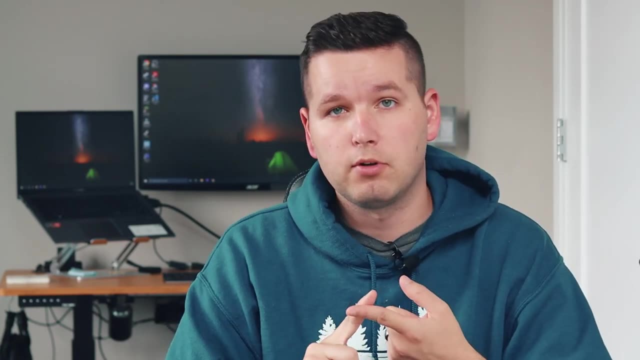 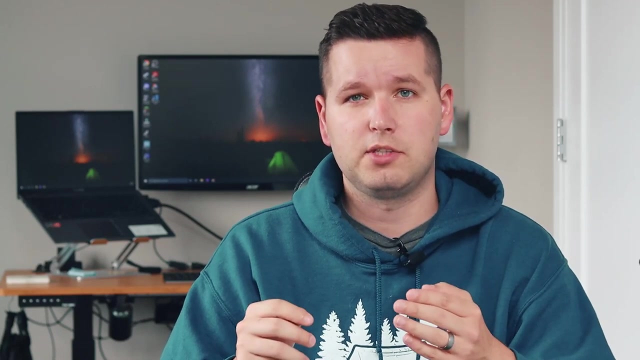 on free RTOS. there's obviously other ones. you could also do like Linux systems, Linux versions for embedded software. as you're learning about all these concepts- whether it's like all the communication protocols that I listed, GPIOs, so on- you want to learn and develop an understanding how to read electrical schematics. 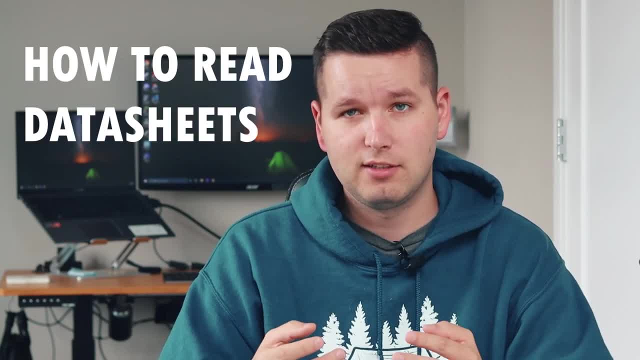 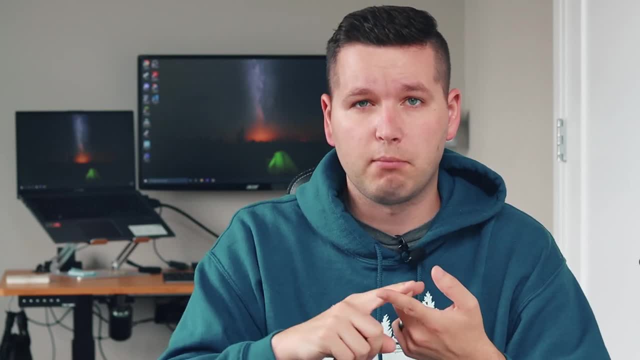 you also want to learn how to read data sheets. those two are very, very important. you want to learn how to you like, use those data sheets, whether it's a data sheet or the microcontroller or the development board that you're using, or if it's a data sheet for the sensor that you're using. 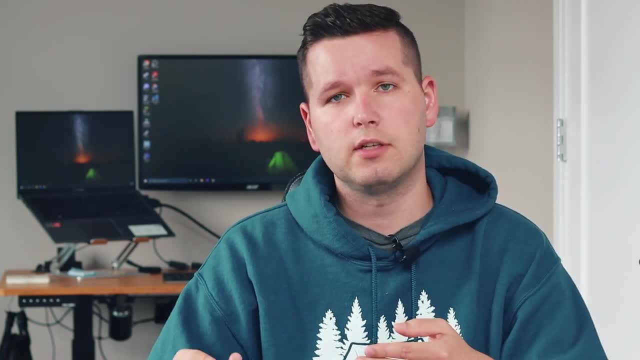 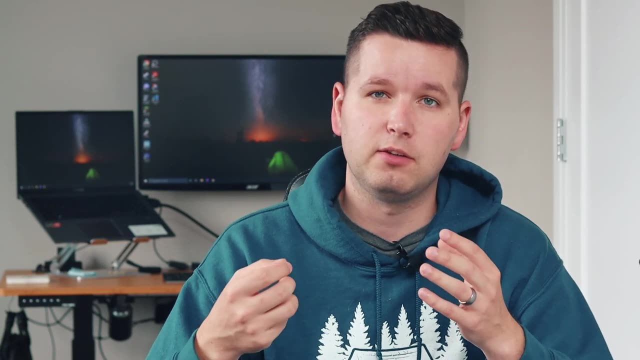 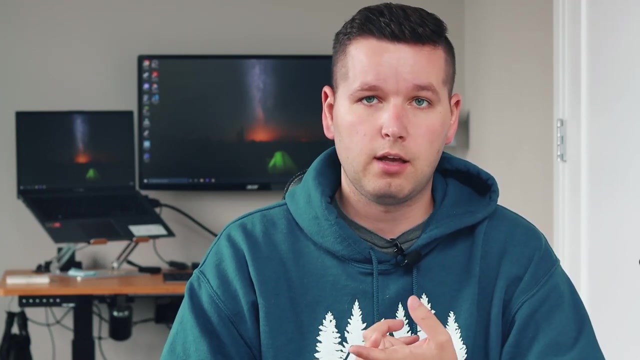 either one of those documents will give you an understanding how the sensor works, how the development board works. you can use that information to write the code properly based on what's given you in that documentation. there are also api documentation that you might want to use, for example, like bluetooth might have api libraries, usb might have api libraries and you can take. 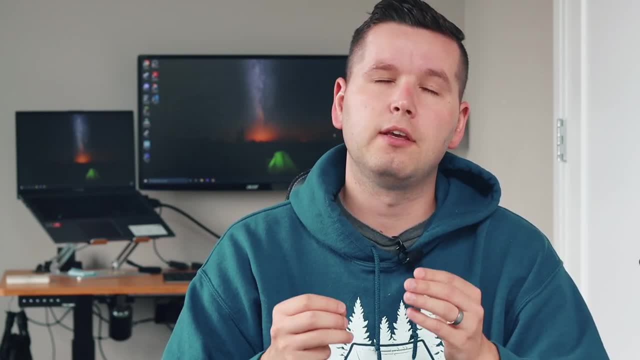 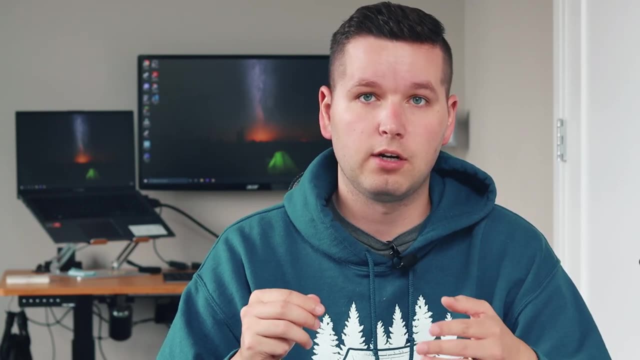 advantage of those api documentations. so definitely learn to handle the documentation i. i can't emphasis this enough- a lot of people who actually start off initially they have no clue how to start off with the api documentation. they have no clue how to start off with the api documentation. 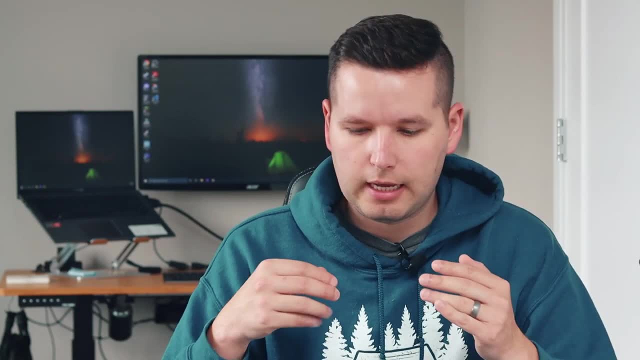 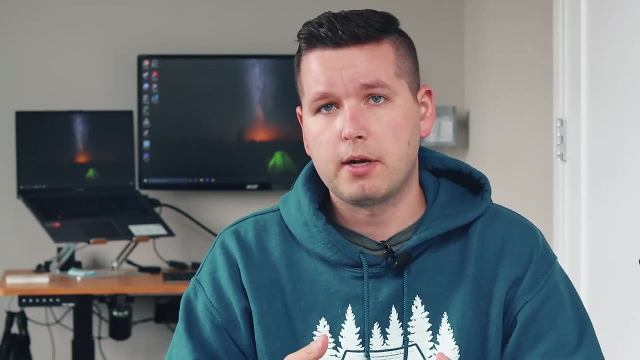 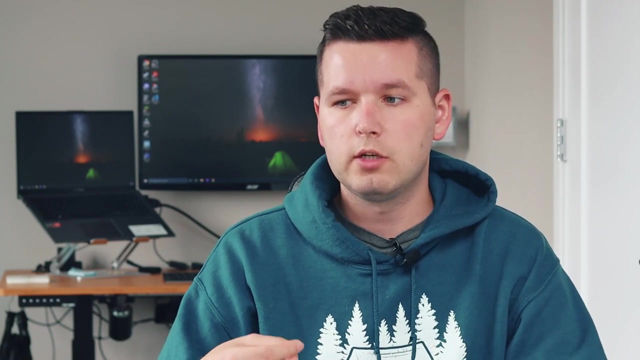 search for things in the documentation. i just wanted to mention as a side note kind of that there are various embedded software engineering positions all around the world and some embedded software engineers are highly involved on the hardware level and they might even give suggestions to hardware engineers on what to put on the new pcba board or how to change. 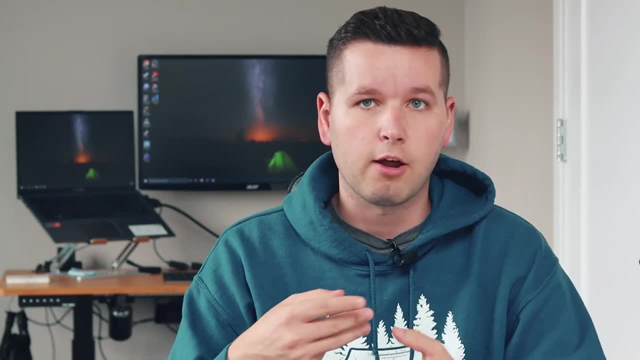 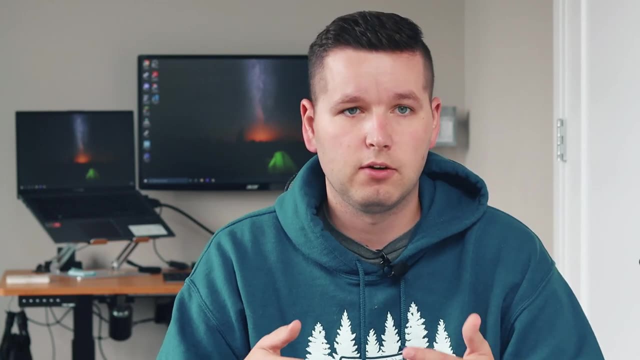 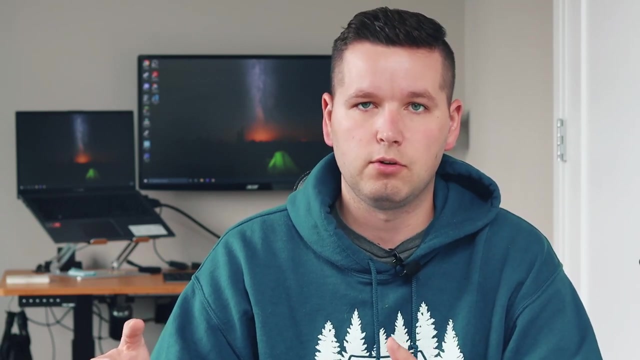 and optimize the board and they they know how to do, like analog filtering and like all these stuff. on the other hand, and there might be embedded software engineers who barely do anything on the hardware side, or, like they, they never, might not even touch the hardware, so it might be like a virtual environment that they work on. what i'm trying to say is: 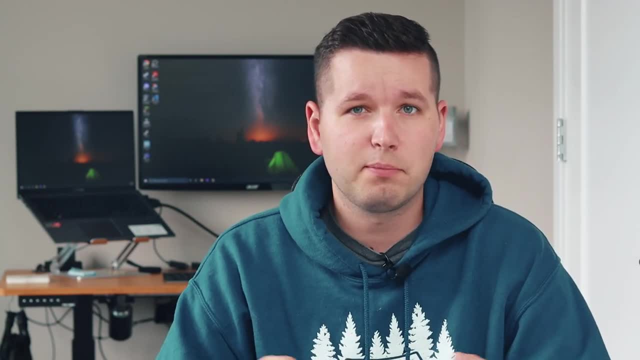 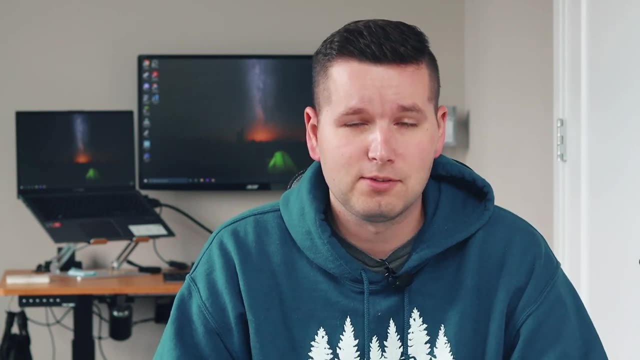 you don't need to know how all the hardware works. i personally don't, and that that is fine. most of my work is done in writing: software doing, god reviews and documentation. as you keep going, you just want to keep practicing and learning new things. there's so many projects you can. 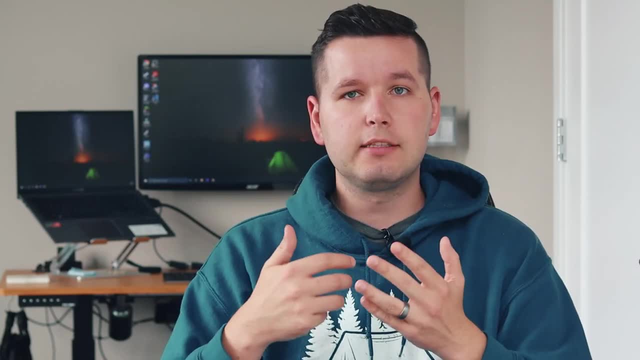 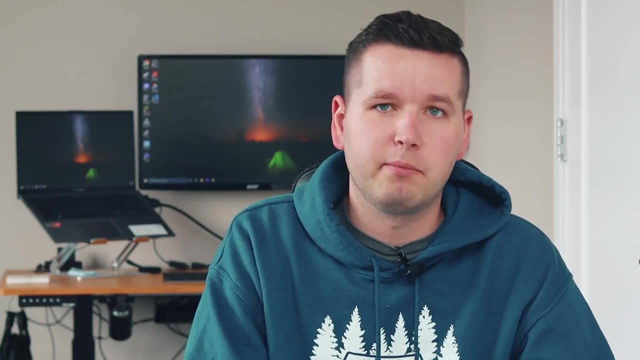 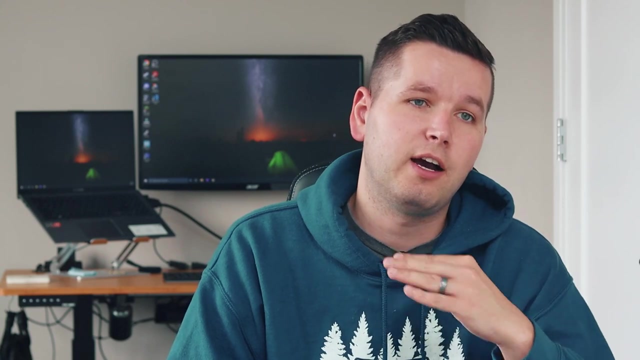 do. there's so many more sensors- and just become less dependent on tutorials. look for inspiration from, like youtube videos, things that other people have done in the past. keep adding more sensors and do some data processing. learn about algorithms. there's a lot of advanced concepts and i highly 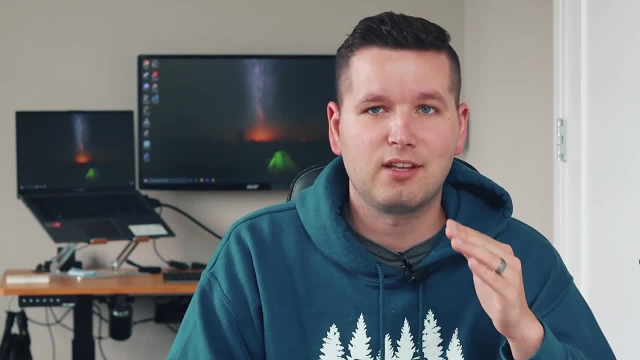 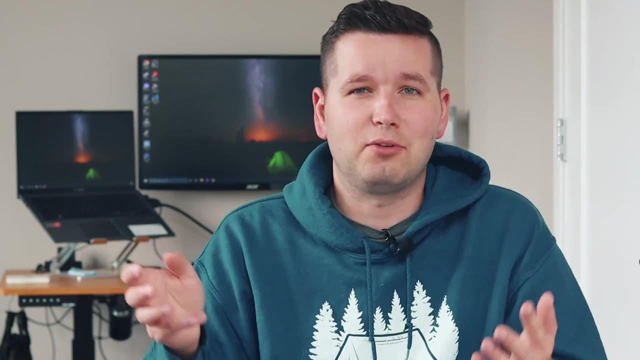 recommend you for to dig into it and just have fun. enjoy learning. i have to break it to you, but knowing how to code and program embedded software doesn't make you an embedded software engineer. you just have to do some of it and if you do that you'll be able to learn all these other techniques.